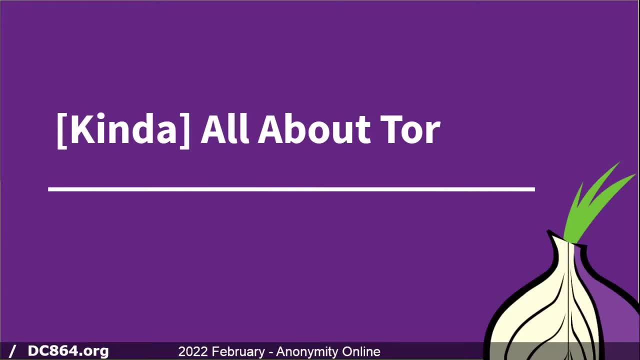 We're not going to go into every nuance and aspect of about it this month, but in coming months we will explore all the different things like relays and running services and things like that. The one thing we want to point out here, and I'm going to say it: 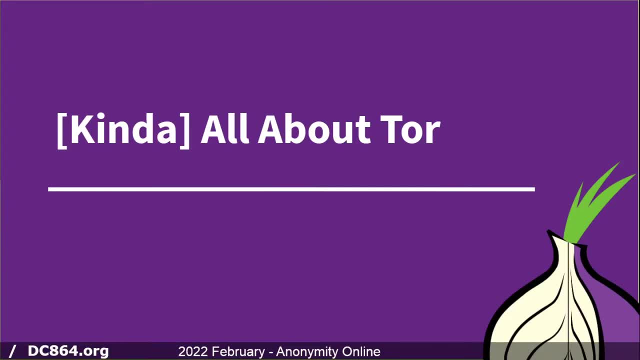 several times throughout this process- is that at no point of what we'll talk about, what I'll talk about in this meeting, or any of the future meetings, is to communicate or convey any type of sketchy or illegal behavior that we're going to advocate online. 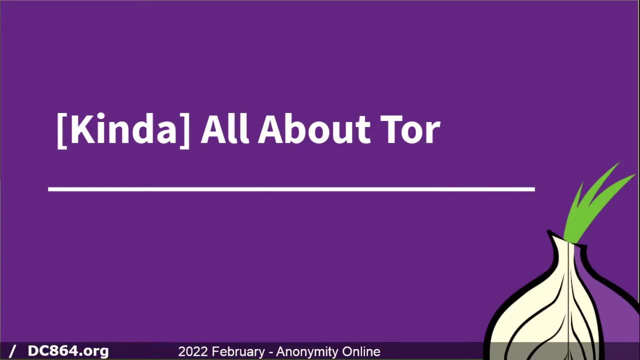 That's just. that's not how we roll or operate as DEF CON 864, but we do understand that we as individual humans have certain inalienable rights and we want to protect and preserve those and how we conduct ourselves online. Before I get started, 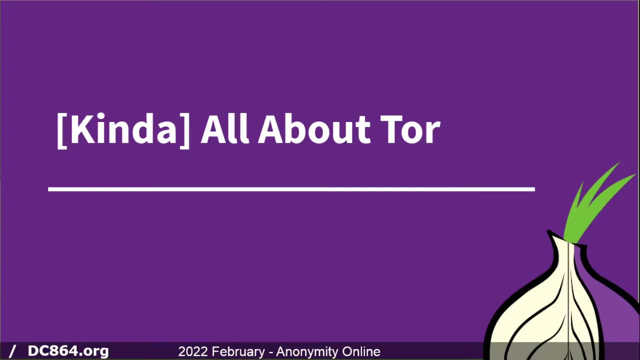 I need to say a disclaimer, and that is everything that I. I'm about to say, apparently, after this point is are my own thoughts, They're my own expressions. They are not those of my employer, either legally or through implication. my spouse. 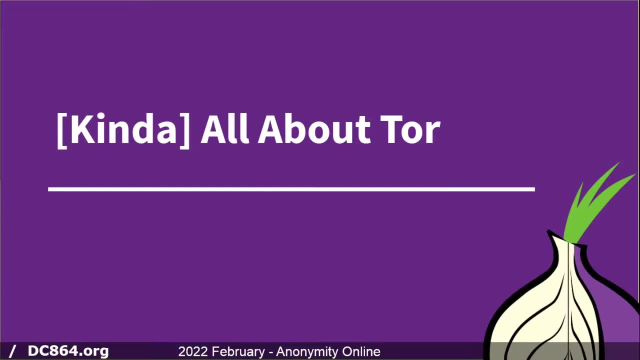 my family, my friends, any pets that I've owned or been friends with, or any code that I have written in the past. So it's all me here, And by saying that, I'm now pointing to a slide deck that I did not create from scratch. 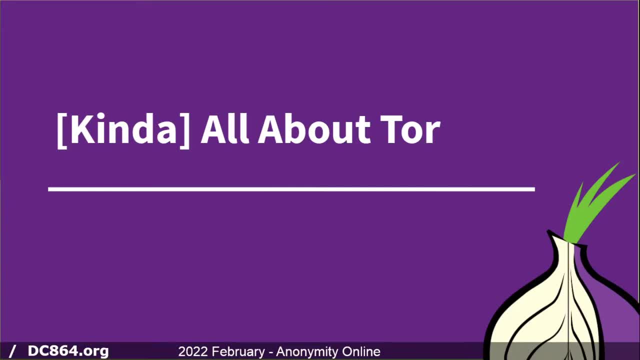 This was put together by the Tor project to help spread the word about what Tor is and help remove a lot of the myth and mysticism around. you know you often hear the dark web and the deep web and Tor. We're going to look into what that is tonight from a high level. 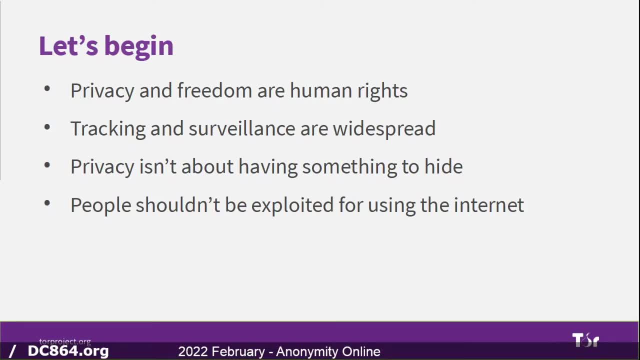 So, at a base perspective, when we talk about privacy and anonymity online, we need to first establish that some basic ground rules and that is just be a good human. So that's one of the core tenants when you talk about a code of conduct for our meetings. 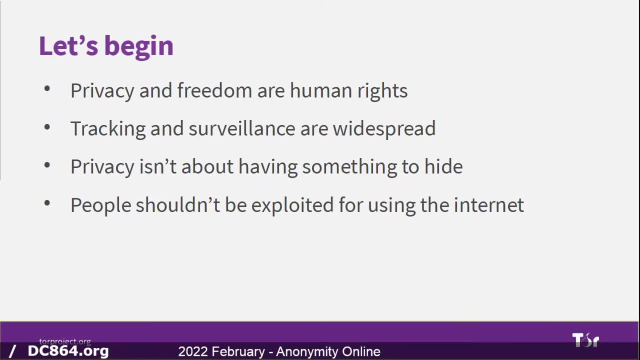 right. We have a thing, that slide presentation, that goes through a little bit and it talks about some nice things, but the the core part of it is to just be nice to other people. The awesome right. So everybody has privacy and freedom as a basic human. 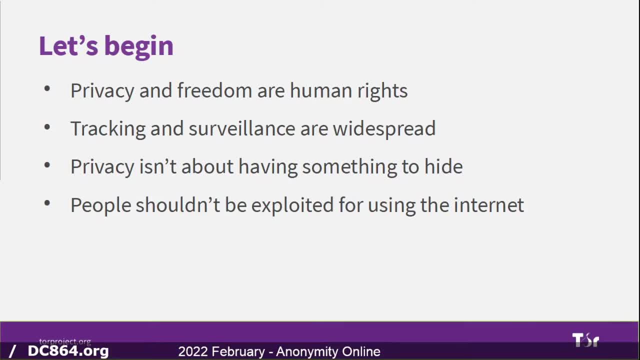 right, But we live in a world that has tracking and surveillance. That's why it's spread, both from a government perspective as well as just from advertising agencies and services that are offered for free and then collected behind the scenes and sold off to the highest bidders. 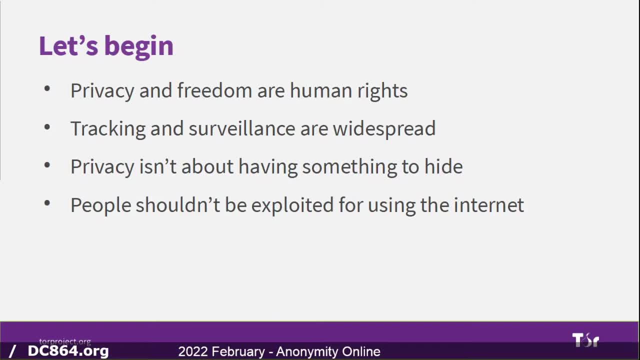 One thing that comes up anytime you talk about using Tor or privacy or anonymity- and I don't know if you've heard this or not, I've heard it from at least half a dozen people- is: I don't have anything to hide, Therefore. 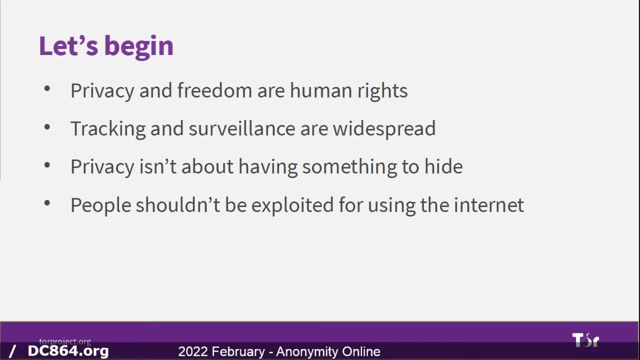 I don't have anything I need to worry about, and that's really not what this discussion is about. It's not what we're addressing. by giving things away by default or living in a society where it's collected by default may set you up 10,. 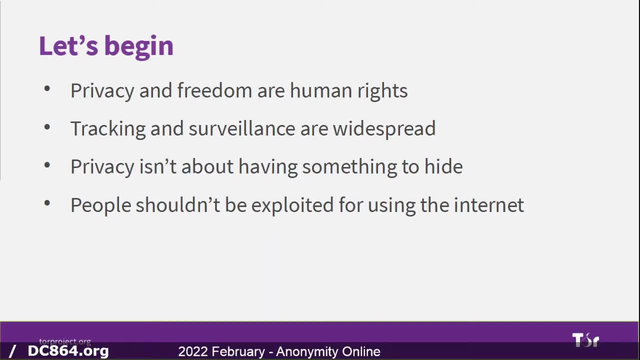 20 years from now, where something that you searched, researched for extended period of time comes back to bite you when that data is collected by your future insurance provider. And now your rates go up and you really have no understanding as to why that is. bottom line is: people shouldn't be exploited for 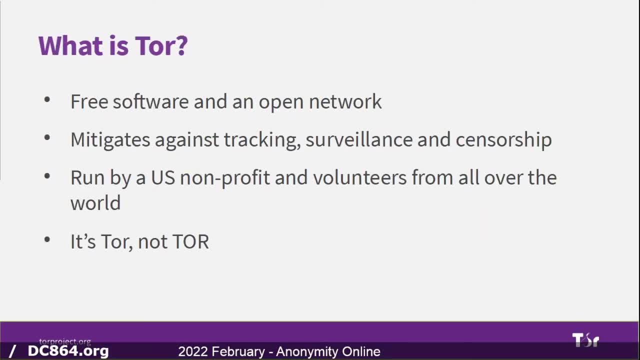 Using the Internet. So what is Tor at a high level? It's just free software. It's open source software and it's also an open network. It's a- it's a tunnel, encrypted network on the open public Internet. It mitigates any risk that we have. 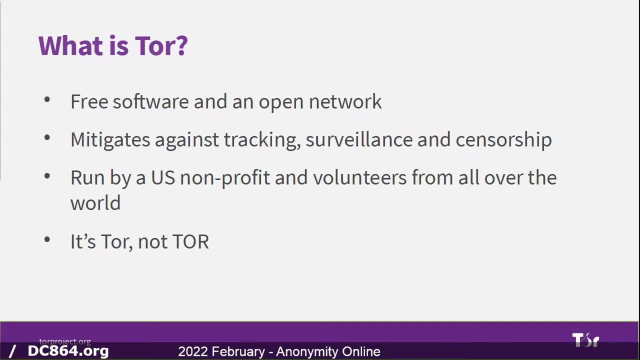 and I say that with a qualifier of being trapped and surveilled in our online activity, as well as a segment for censorship, which we're not really going to get into tonight too much. But if you're in a country that censors Internet activity running, 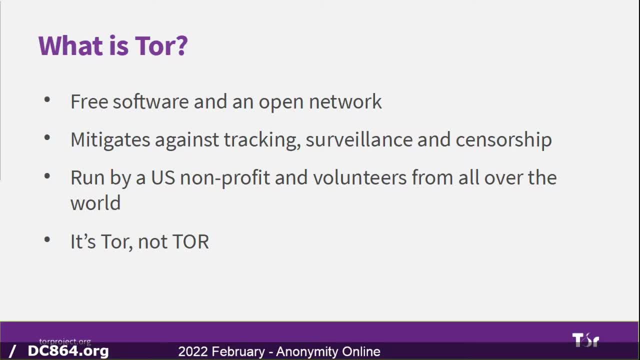 and and using Tor can help you get around that. censorship is a caveat. I want to point out here that I'm not advocating in any way, shape or form that you download and install Tor on your work computer, on your school computers, like that's a great way of getting an interview with if your organization is mature enough. 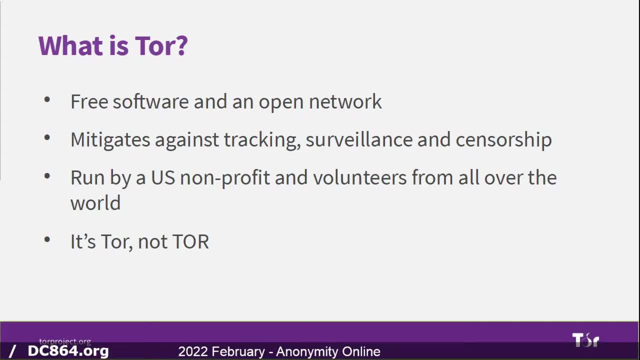 That's a great way of getting an interview with people you don't want to really be getting on the radar for Right, So we want to be playing nice in that realm. But when it comes to us as individual people, we don't necessarily have the same protections that our corporation does in isolating their network from the public Internet. 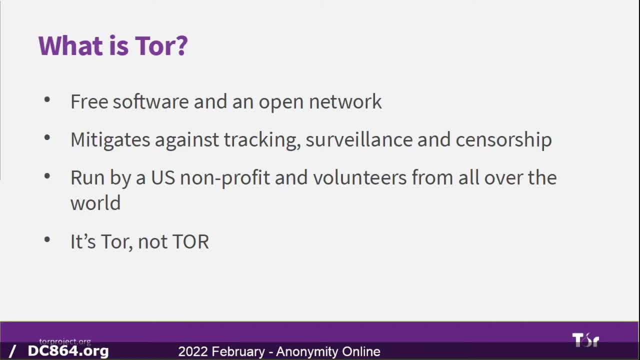 Right, There's two points, Parts of what is meant by Tor and the Tor project. There is a US based nonprofit company called the Tor project and then they oversee the software that's released and put out. It was originally created and started by the US Navy. 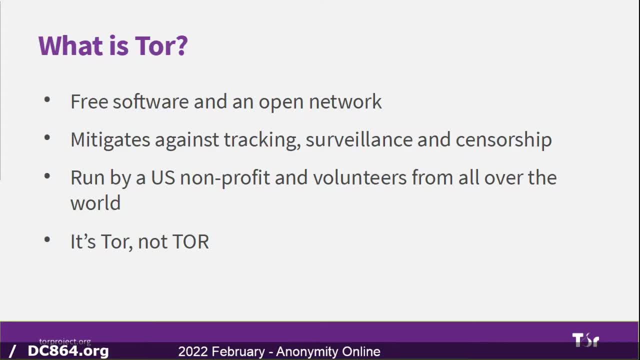 but that's long since been turned over to this organization. The code is open source. We can all read it, read through it and dissect it, And each of us could run relays on the public Internet to basically build out that Tor network for everyone else to use. 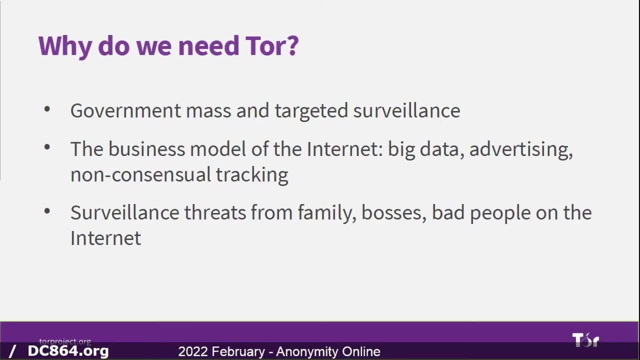 So it's run by us. common people Pretty well understood that, everything from the services that we use for email all the way up to the governments that are protecting us- And I'm air quoting that extensively within my head that they're all tracking us and keeping track of what we do- 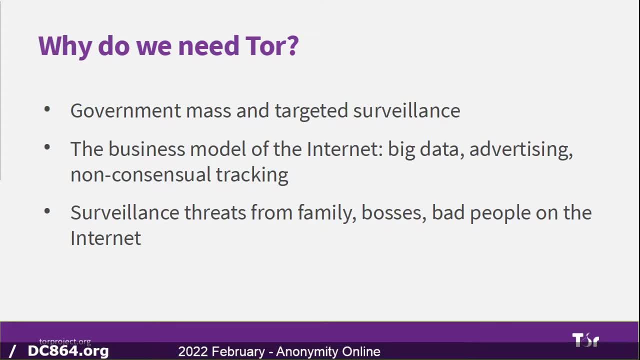 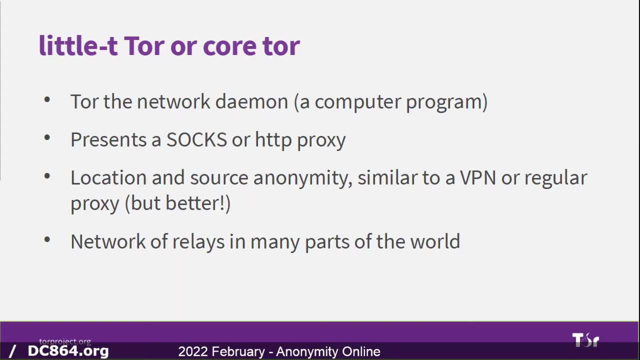 So surveillance. threats come from many different locations, not necessarily just evil actors online. So there's two parts to this and how it completes out. You have the Tor browser, which connects to the Tor network through a network daemon, which, if you're a Linux fan and you've been using Linux for a while. 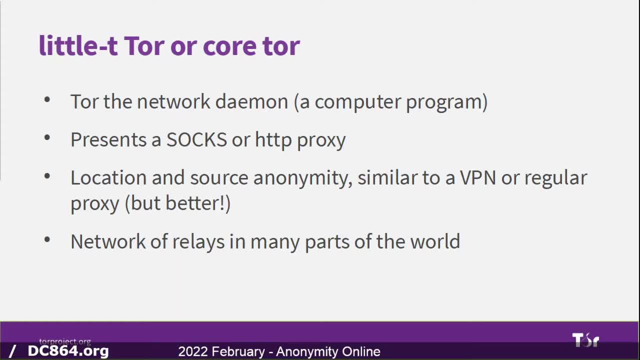 you're pretty familiar with daemons, but it's really just a computer program that runs almost as a service and it presents a SOX or HTTP proxy. It defaults to SOX, but it has some fallbacks and location and source anonymity. We get into this a little bit more in depth later on. 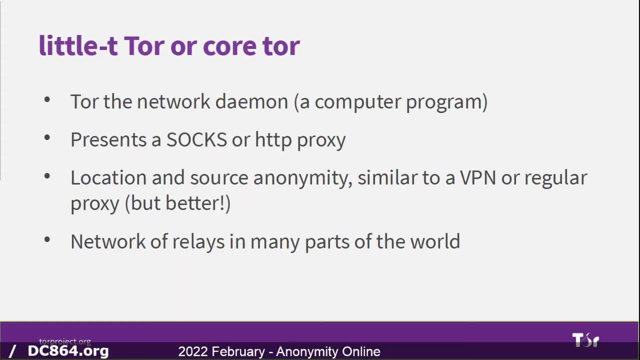 but this is really important- where you're searching from your laptop. Your PC now gets hidden and isolated away when you use Tor and it's now sheltered through that Tor network. So what your traffic comes out the other side is now looking like it comes from the big, nebulous cloud of Tor, as opposed to your home ISP. 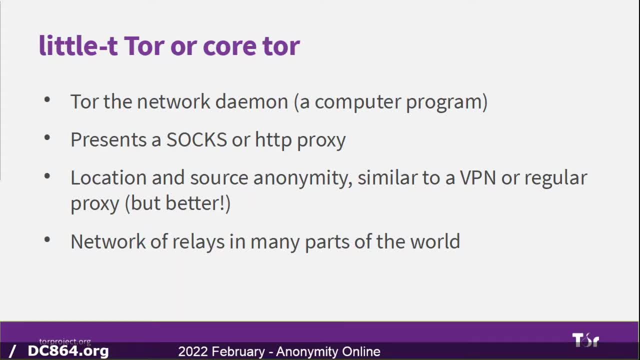 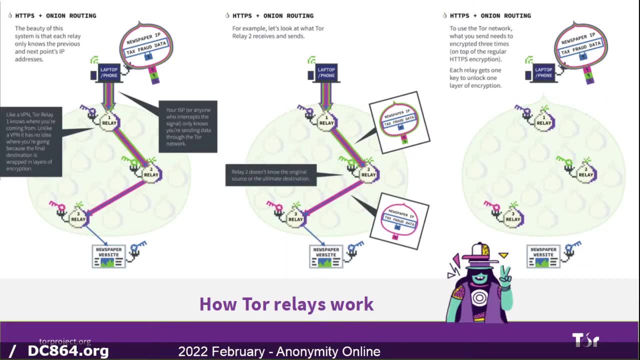 And there's network relays in many parts of the world. I think the last count it was over 6,000 relays around the world. Basically, there's a really intricate process for how the data is encrypted. We often think of encrypting internet traffic with HTTPS. 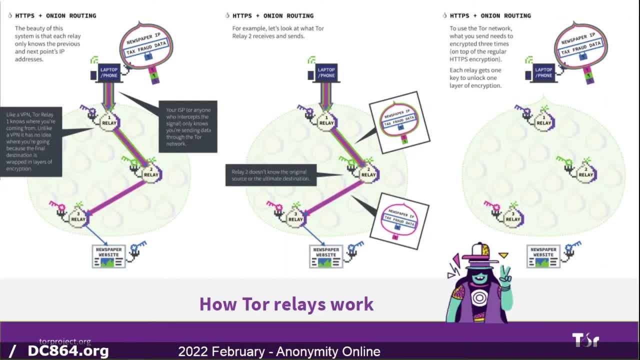 where we're just securing that transport layer to make sure that nobody's really listening in to us. But if you look in the top left you have the onion, and Tor stands for the onion router, And so it takes your data that you want to search the internet for. 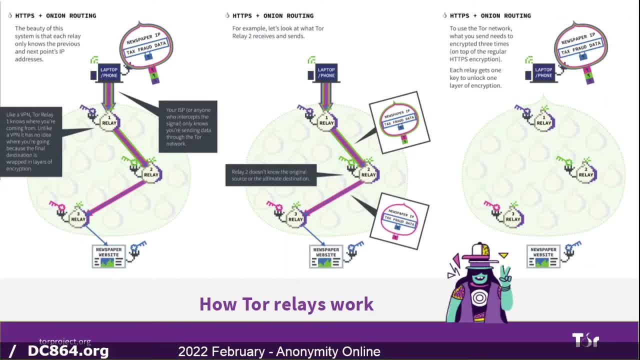 and it wraps it in three layers of encryption using three different keys, And those keys are known by- and it's a Diffie-Hellman encryption. for those of you that want to geek out over that, Those three layers are intended for three different nodes in the cloud of the Tor network. 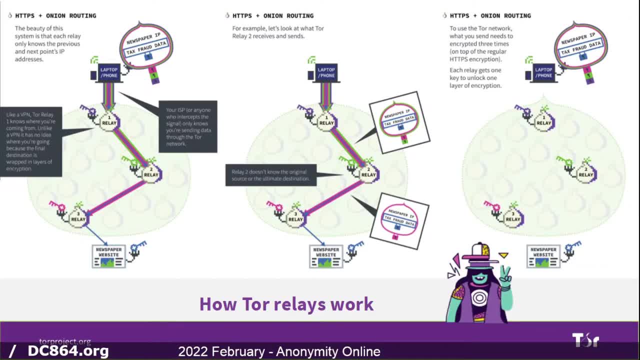 In order to get those keys and know how to do that encryption, the Tor browser first queries a directory server similar to DNS. It gets that listing of what it's going to use and it picks three random nodes, three random relays in that connection. 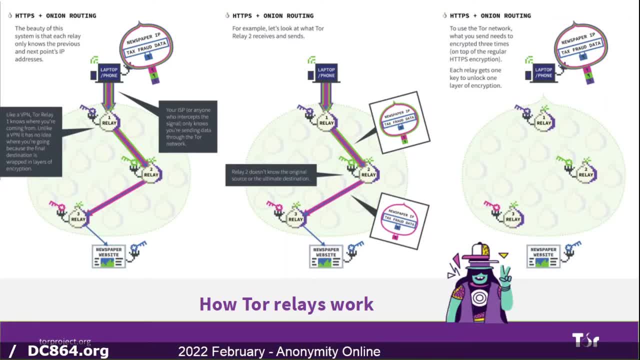 and then builds your packet to go through that And as it passes through each one of those relays, the encryption layer is stripped off, passed to the next one, stripped off, And then when it hits that third relay, that's called an exit node or an exit relay. 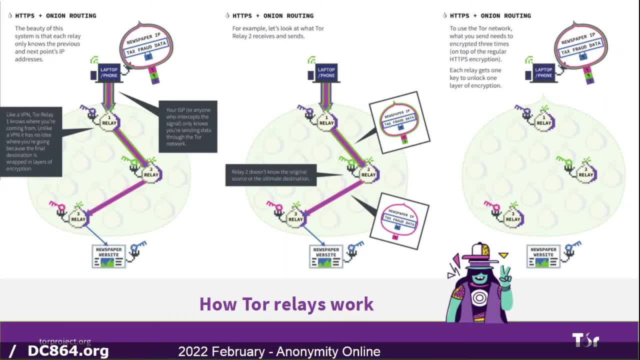 And that final layer of Tor encryption is pulled off and it's now just HTTPS going out over the public internet to your destination. So anything in that Tor relay, that Tor scenario, that Tor cloud there, that Tor bubble, doesn't know what your data is. 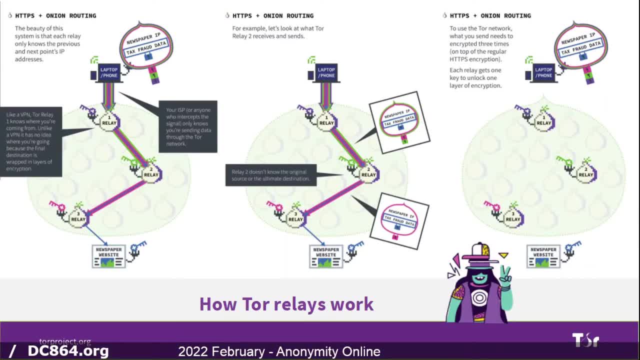 It doesn't have access to that. At most it knows the relay or your source before it and the one after it. That's all it knows. It just knows source and destination in those places. So to look at that in depth: 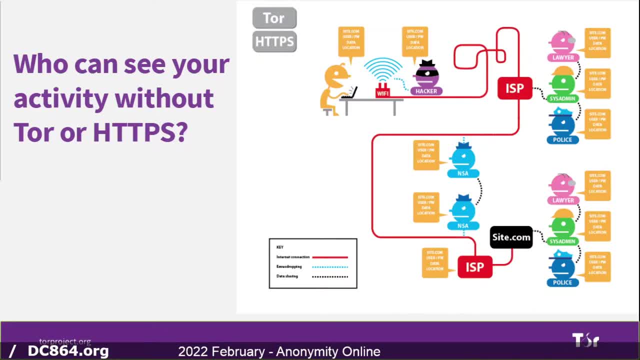 if we take a look at our standard use of the internet today, when we don't use HTTPS and we don't use Tor, everything even if you have a hacker sitting on your local network, they're watching your traffic. So, if you notice, in the top left. 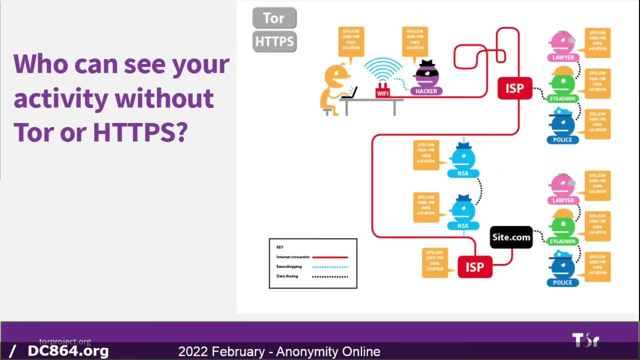 you've got this person sitting in a laptop and it says sitecom user password, data and location. That's all the data elements that could be collected for a fingerprint that would identify that individual uniquely on the public internet And by default when you send that over the wire. 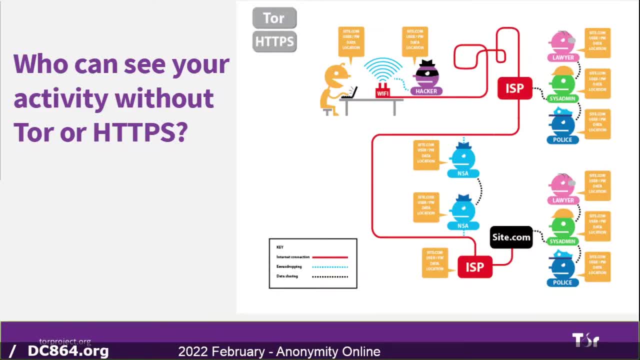 everybody in the food chain, from your ISP, everybody that they want to sell that data off to, to the intelligence services that are working with those ISPs to monitor that traffic. all those people have access to that information and that data And it flows all the way down to the site that's getting it passed over. 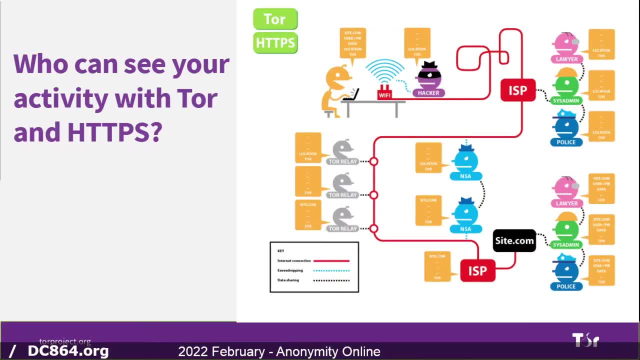 Now you can see, if we move over to the next slide, who can see your data and activity with Tor and HTTPS enabled, And you'll notice that the bubbles for each of the players in between you, the source and your destination at the end. 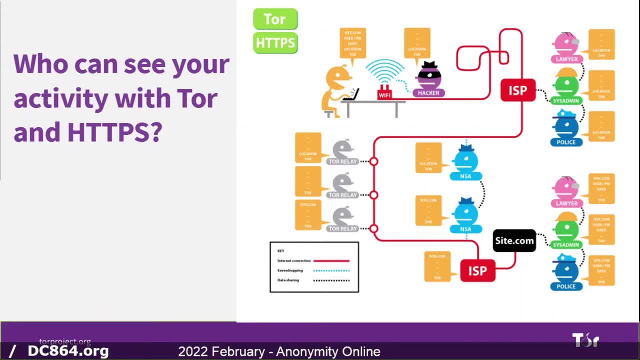 that's sitecom. all of a sudden those data values start to disappear and they get blanked out. They can piece together individual aspects of that data, but they can't put together the full picture. And most of these marketing companies, advertising agencies, 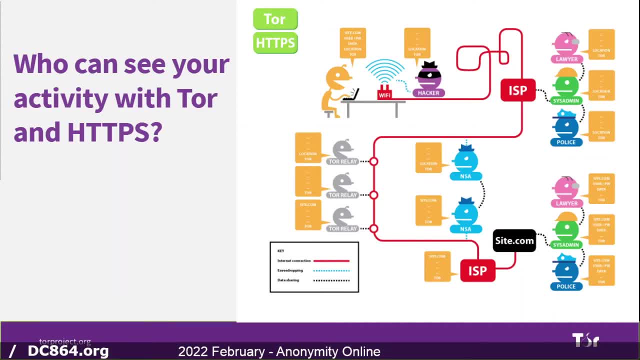 what they're hoping to do when they're gathering up all this collected information is find unique ways to identify your unique fingerprint on the internet- Everything from the resolution display of your monitor, like all kinds of unique things that they can do, Like in the last week. 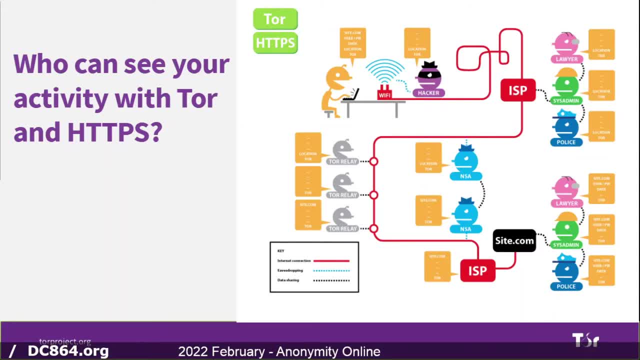 there was a new fingerprinting method that was just published out, and I'm going to draw a blank on what the name of it was, but it uses your GPU and JavaScript right to calculate a unique fingerprint ID, Even if you have the exact same graphics card. 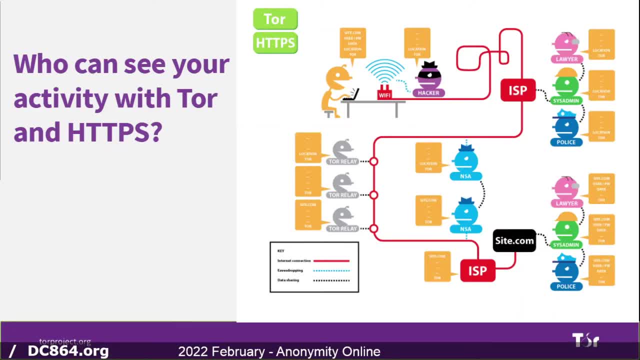 like if we had the exact same graphic card. we have two unique fingerprints as a result of that calculation, So that's a new one to watch out for. But in this scenario here, what we've done is we're basically just tunneling all of our data. 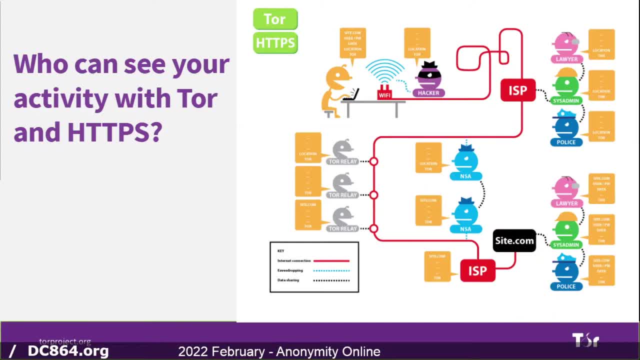 and shuttling it across the Tor network and isolating away from all of those people's eyes. And this is typically where somebody would throw out the statement of: well, I don't really have anything to hide, so I don't necessarily care if they monitor that. 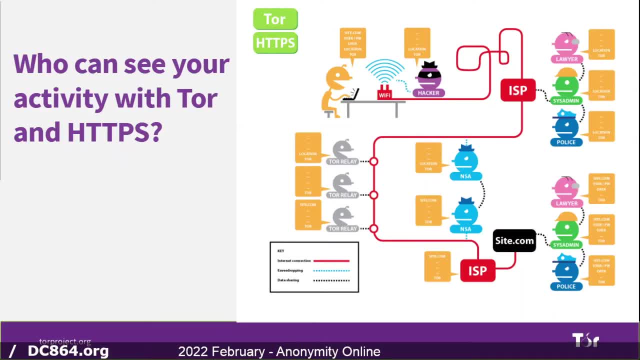 But you're assuming that all those people between you and that site are altruistic or transparent in what they're doing with your data, That they don't have any other purpose for using you uniquely to fit some other means. It's not a two-way street here. 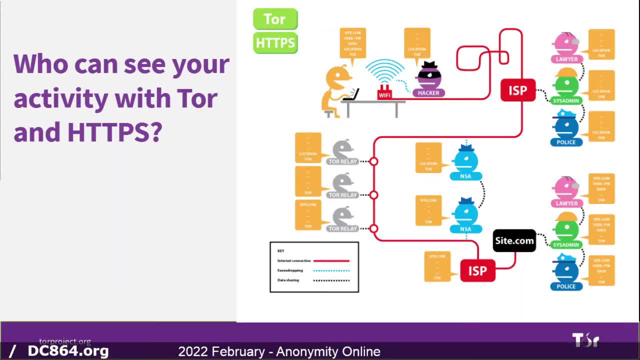 It's not an equal anonymity scenario, Each of those watchers, between the ISPs as well as the companies that they sell off to in their collections. they're not up front in public about anything that they're doing. If it wasn't for watchdogs, if it wasn't for whistleblowers. 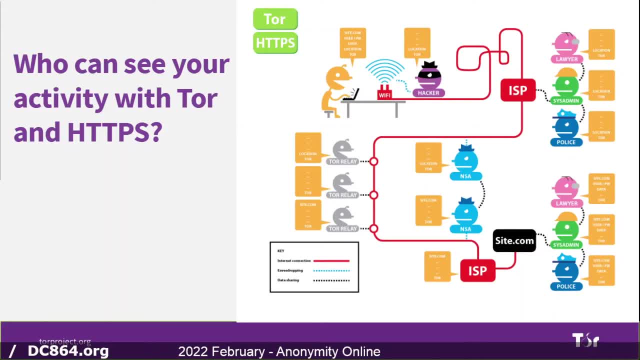 we, the people, wouldn't necessarily know some of the services that are collecting the data on us. So it's not a fair game, right? They want us to be fully transparent online, but they're not necessarily being fully transparent with us. So when we look at the Tor network, 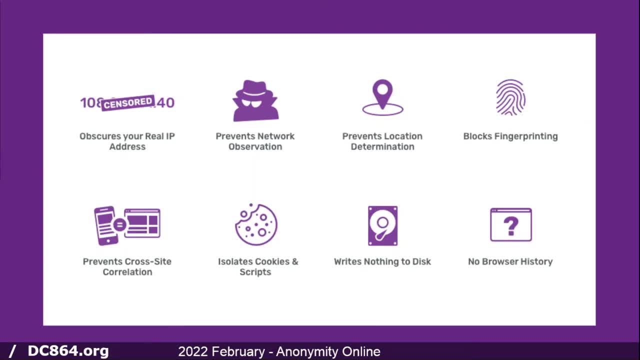 I mentioned that it blocks fingerprinting, and there's just a few examples on here where it hides some of that information about us. So, for example, in the lower left it talks about cross-site correlation. If you have two tabs, the Tor browser does an excellent job. 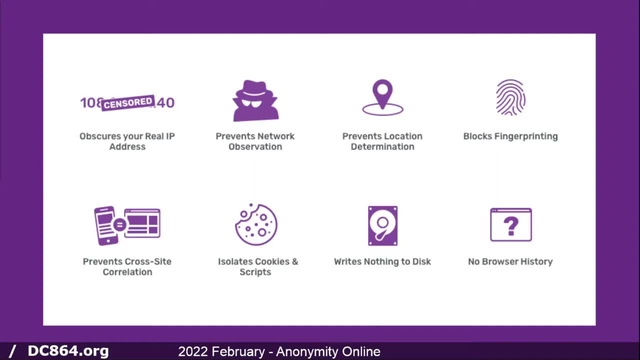 better than any other browser of isolating what communication can take place for the identification of you doing that, browsing between those two tabs, Fully isolated off right. The comment at the bottom where it says writes nothing to disk. I don't necessarily agree with that. 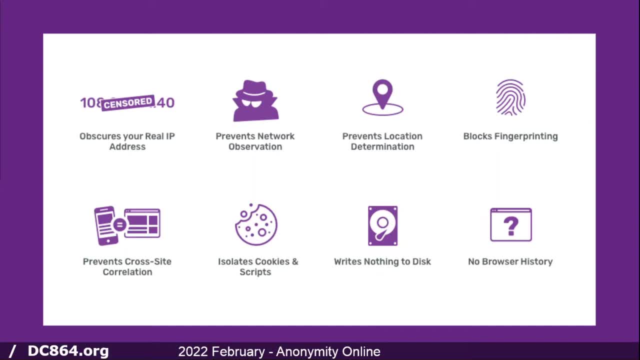 It does write trace information to the disk, but we'll cover in next month how to get around that to where you can have an amnesia-based web presence, And we'll get a little bit into the complexities of what it takes to truly be invisible. 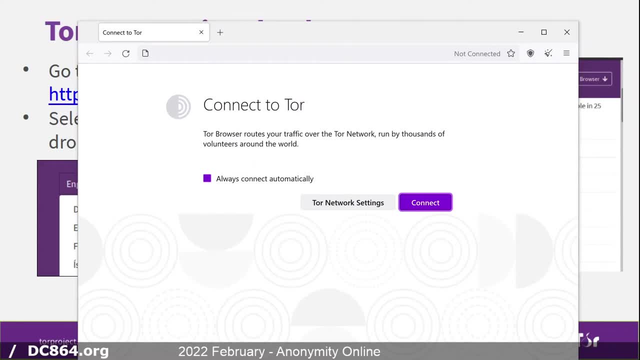 All right, so this is the start page for Tor. When you first load Tor on your system, let's say that you have a standard Windows laptop or a Mac and you're going to install and load the Tor browser. You're okay with using it for research. 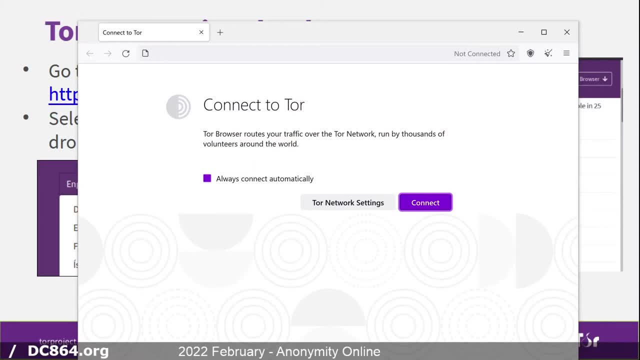 and this is how I normally use it. I like using it as my default browser. It defaults to have two plug-ins enabled by default, That is, NoScript and HTTPS Everywhere. So if any site tries to do that, to downgrade you to HTTP. 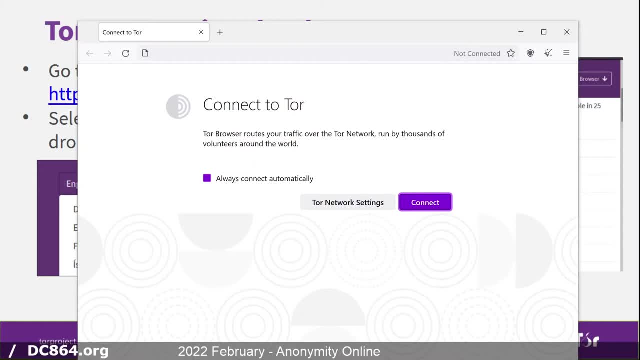 that's getting forged up to HTTPS. If a site tries to load a bunch of JavaScript and reference other sites to load their JavaScript, I mean potentially that's a supply chain attack, right. But on this base site here, what we're looking at here? 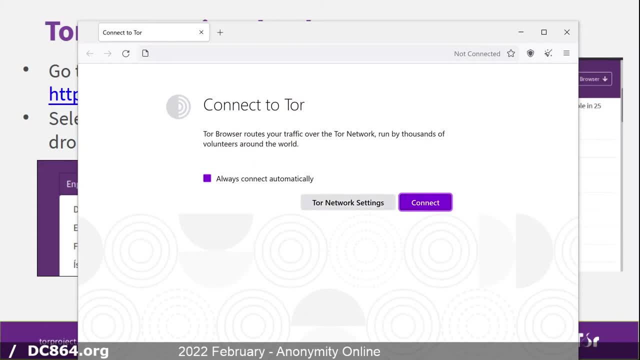 it says connect to Tor and you have two options. Well, a couple options. right, You can look at the settings, which we always do as security professionals. The first thing we do is look at our settings to make sure that they meet our operational security needs. 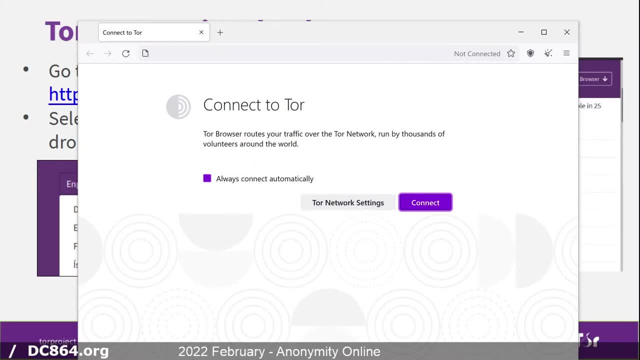 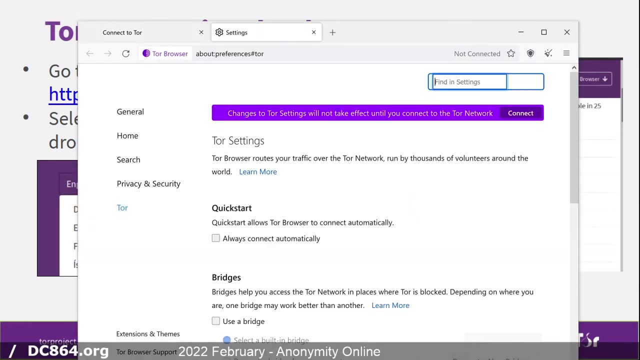 and then we connect to some network. here You can flag the box for always connect automatically. This is if you didn't necessarily want to always be on Tor when you fired up the Tor browser. If I open up the Tor settings, you'll notice that. 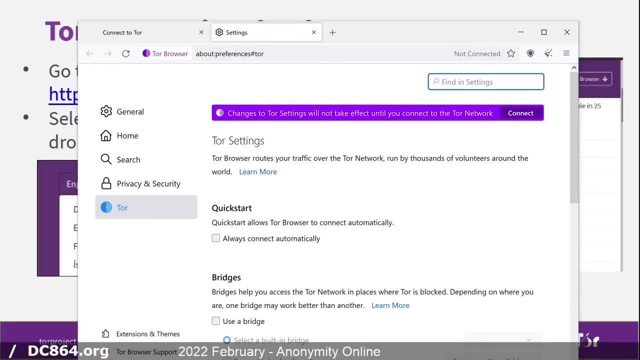 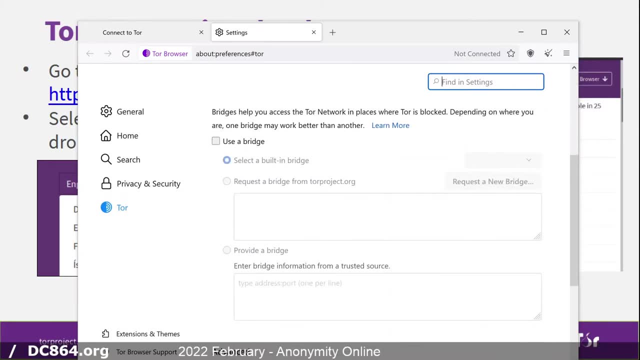 and this is a build of Firefox, by the way. so if you're used to using Firefox, it's the exact same. You just gain some extra parameters and settings under this Tor setting here, The one that is of most interest to you. 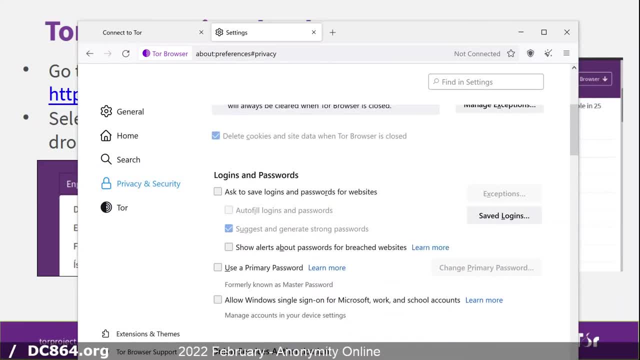 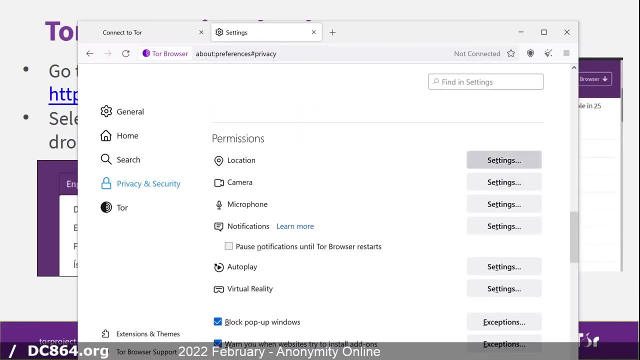 if you go under the security and privacy setting, there's a couple things that I recommend to do. The first is to, For whatever reason, they don't have these disabled by default, like location camera, and otherwise You have to enable block new requests. 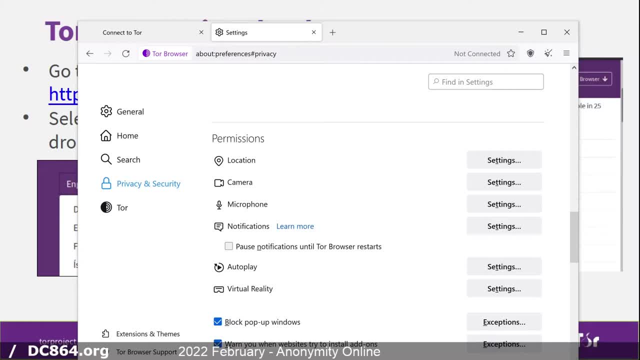 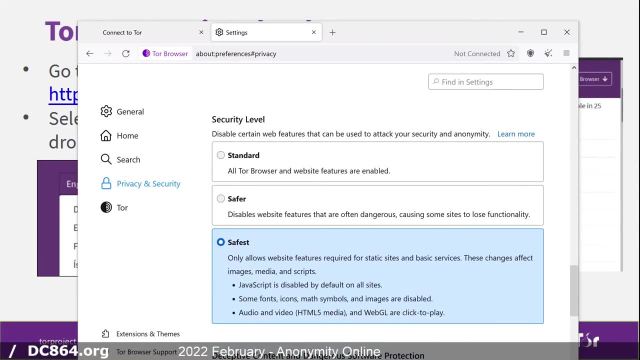 if you wanted to have that in there. So normally when I'm doing my research I don't like anything popping up or asking for any of that. And then at the very bottom, by default it runs in standard mode. That will allow JavaScript and other things to run. 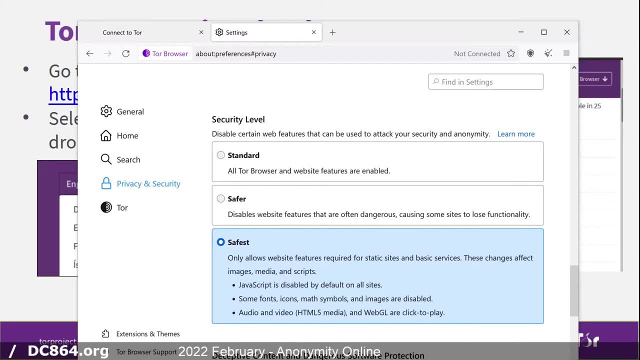 It's dangerous. in that regard, You can go to the safer option. but if you want to be the most efficient in your research, if you're just really down to read and study information, going into safest strips away a lot of the distractions. 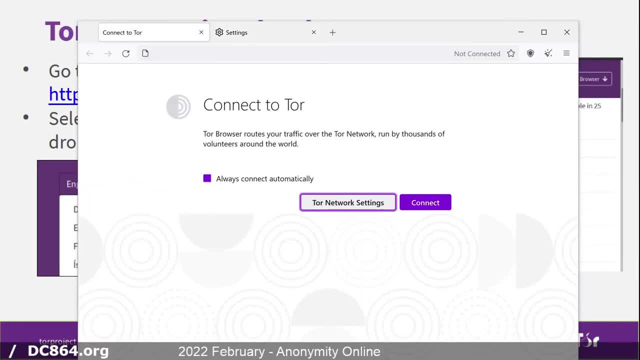 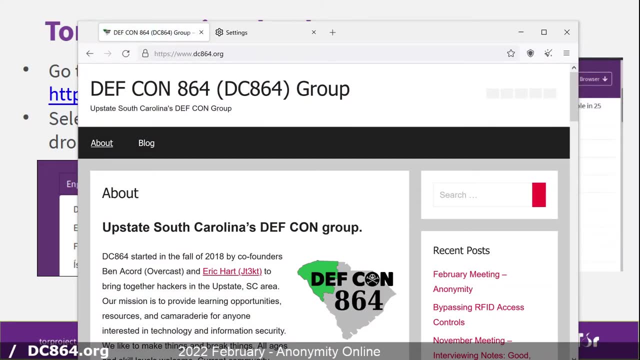 I have this set on safest right now. Let's go back over and connect to the Tor network. All right, so we're establishing a connection. You'll notice that it is slower and that's expected, right? I mean you're basically doing now. 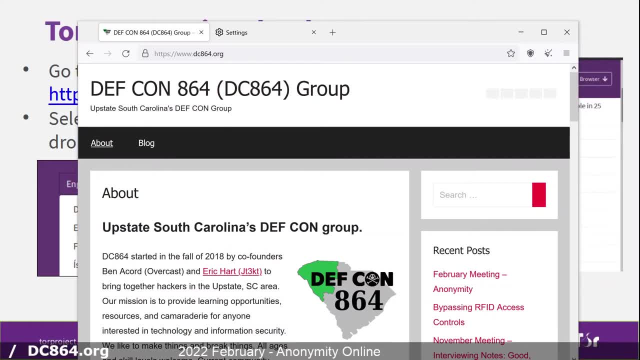 three times the level of transport encryption that you would normally be doing over HTTPS. But up here at the top we have our friend, the padlock icon. but when we click on it we get a lot more information than we normally do with just a certificate. 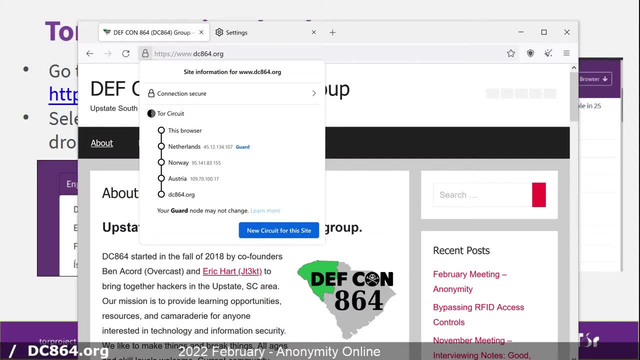 So this shows the circuit that it built for us and how we're navigating around the world in order to reach the dc864.org website. In this case, we're going through the Netherlands, Norway and Austria, One of the things I want to point out. 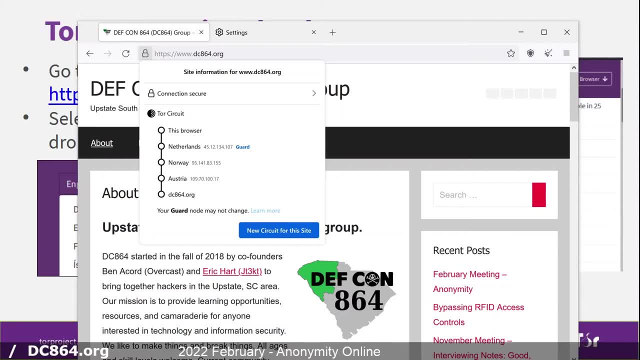 is not all relays are created equal. Some of them actually have special status that we want to highlight and we are going to go into depth in the coming sessions on these. as we look over this first one, the guard relay, You'll see that one stay with you. 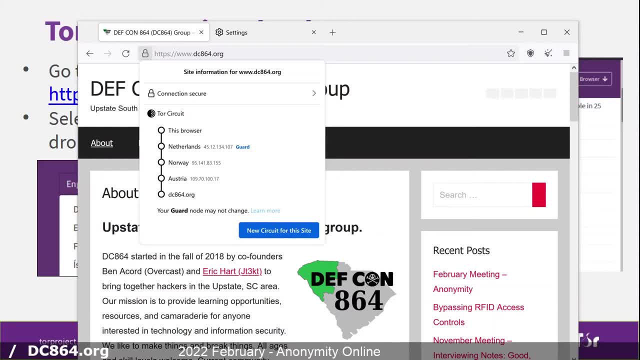 for a longer period of time where, like every 10, 20 minutes or so, if you check your circuit, you'll notice that these other two are changing out to something different. So your route through that is never. Data isn't passing through the same relays. 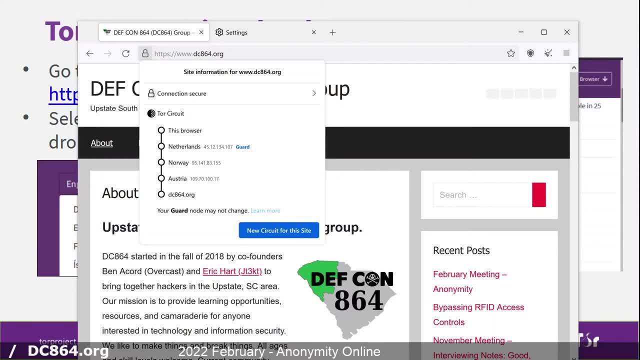 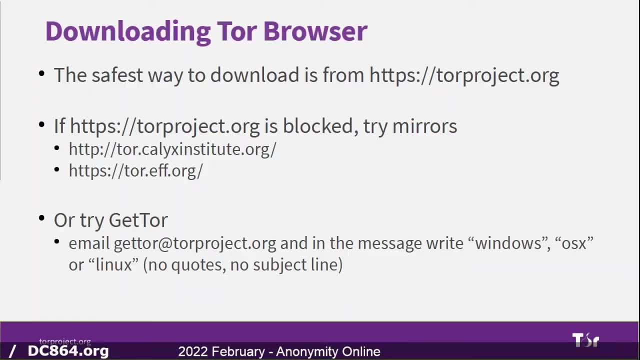 all the time. The longer you surf the web with Tor, the more routes your traffic is going to take to your destinations. So, downloading the browser, you can go to the Tor project site to download it If it's being blocked or you're having difficulty. 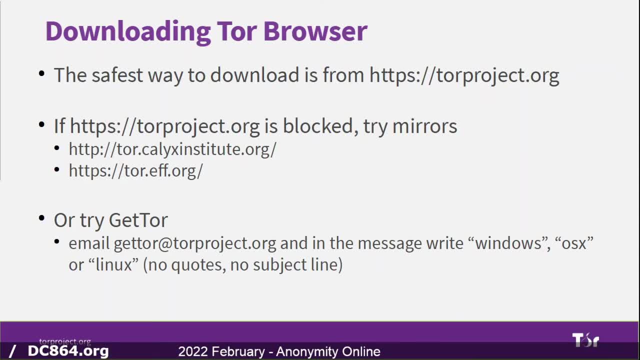 accessing the Tor project site. let's just say they're undergoing a DDoS or a DDoS update. it's going to be a DDoS update and you can download it, And it's going to be a DDoS update. 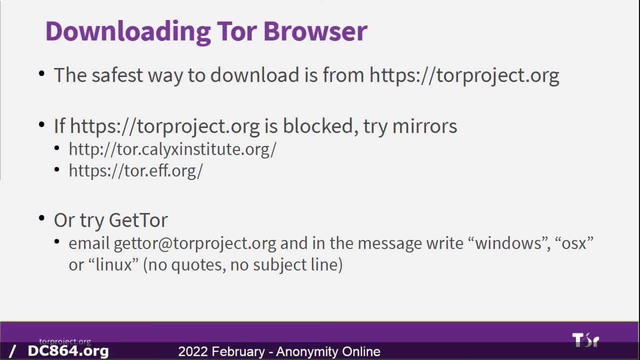 if you have any issues with that, So that's going to be something that you'll be able to do if you're having trouble accessing the Tor project site. So the next one I would like to talk about is a couple of other things. One of them is the DDoS update. 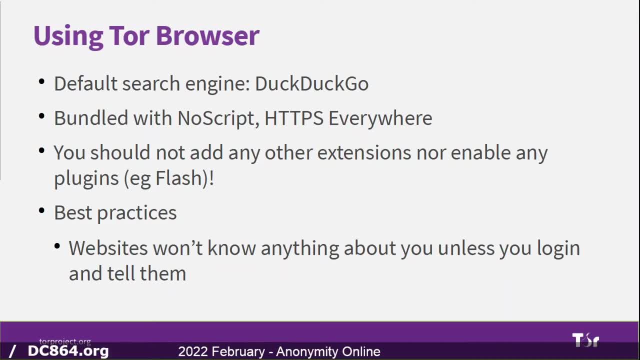 So if you don't have a DDoS update, you can download the DDoS update and you can use the DDoS update how it's packaged, together with NoScript or HTTPS Anywhere. keep yourself from installing other plugins or extensions into the Tor browser. It says Flash here, but everybody at this. 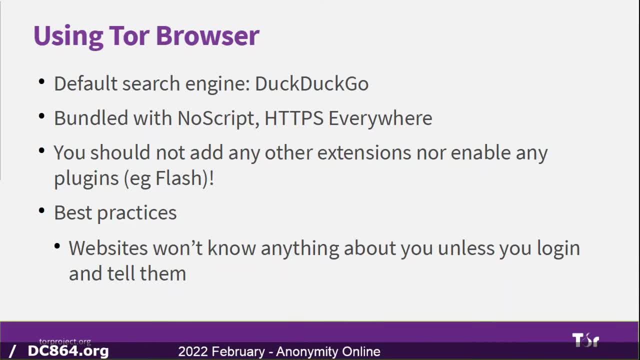 point knows that Flash is a bad idea and we probably should have killed it soon after it was released. Best practice is just use it as vanilla and straight as possible, maybe making some of your offset changes in the settings, But other than that, just keep it. 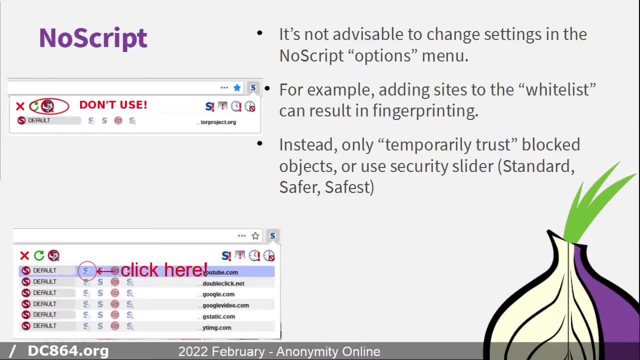 as vanilla as possible. So this is an example of NoScript. For those of you that haven't used NoScript or aren't familiar with it, in the top right of your address bar you would see a pop-up that would indicate the number of sites that are requesting to run. 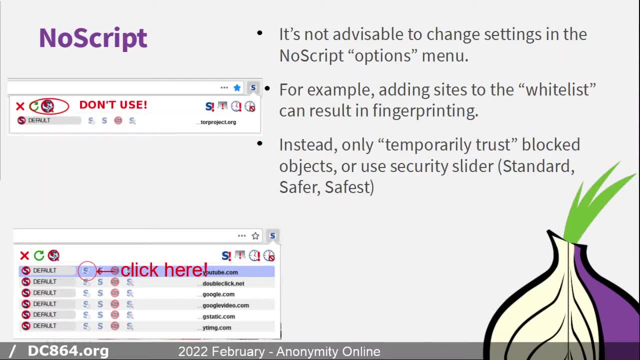 JavaScript in that browser section So you'll see that number tally up. So in the case of the first item up here, it would just be one, And so if you click that item to come down, we never want to use the global whitelisting approvals for JavaScript. We always want to. 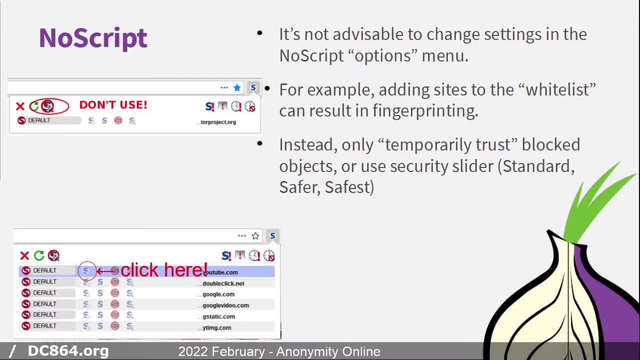 use the temporary approvals for JavaScript within Tor browser, And the reason why is: the more you customize and change it, the more you're basically creating an identifier of who you are in that browser section. right, And that's the same reason why to not install extensions as well, because those 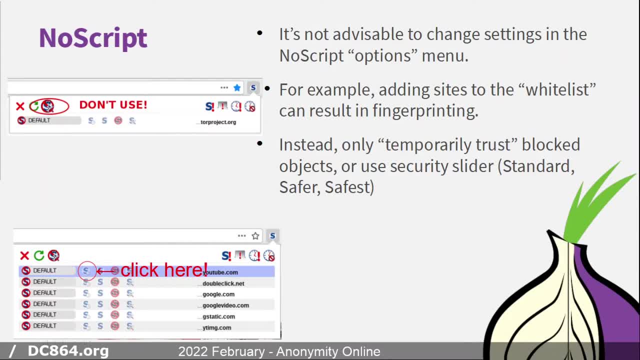 things can be used for anything. You want to stay as plain as possible. Exactly, And if we are whitelisting these sites to run JavaScript in our browser and then, like I talked about, they get supply chain breached? now we've whitelisted and 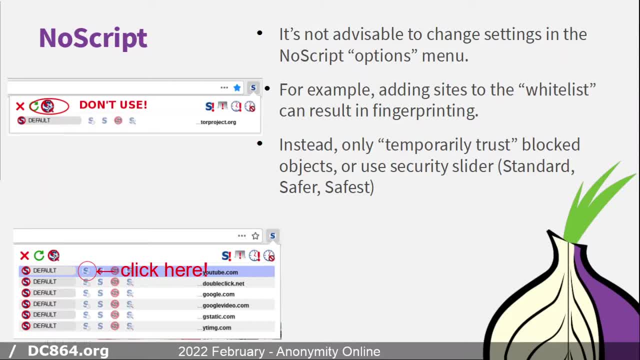 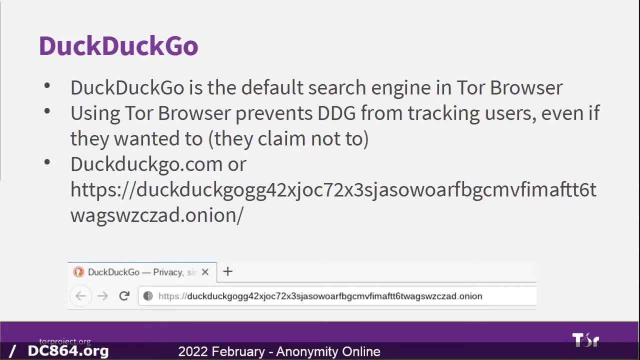 authorized that site as a trusted site and now they're just running any JavaScript They want as well. And the same thing with extensions. The DuckDuckGo- is that actually a good browser that protects your data? It is a good search engine. It is not as thorough as Google and we can go into, maybe, how that. 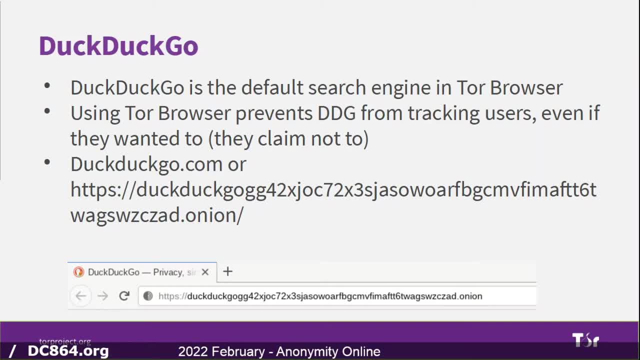 algorithm works. It's intentionally a bit different than Google Now what I'm showing on the screen here as well. DuckDuckGo claims that they don't track you, which is a big win. We want to see those kind of confirmations from companies that we utilize, But at the 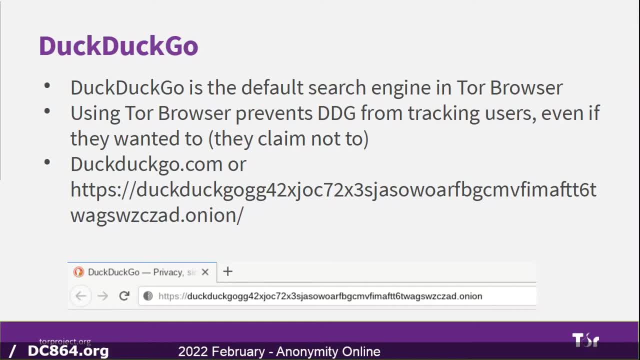 same time, it's nice to have a browser that's enforcing that for us, Right, Even if there's maybe like a leadership change, you know, or something that happens behind the scene where we question what's going on there. at least you know we're. 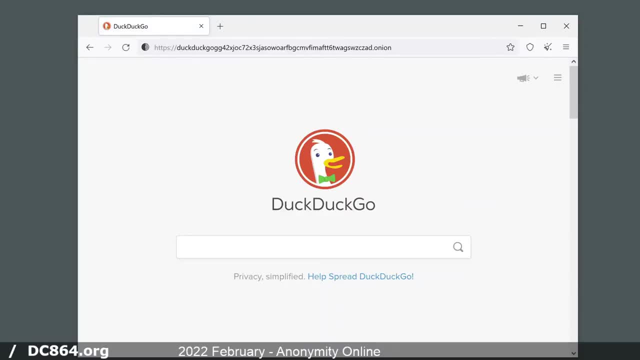 doing our part to make sure that we're secure there. So Onion services and websites have a unique string at the beginning and they're not user friendly. It's not like a DNS resolvable name that's super friendly and easy to use, But 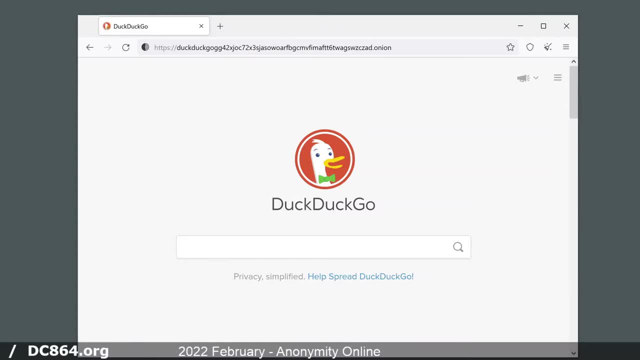 they always end in a onion and that's the addressable space within the Onion network and the Onion router. One last comment: So I've spoken a lot about using Tor with a, you know, a laptop, a PC, more of a physical endpoint that's more substantial right There. 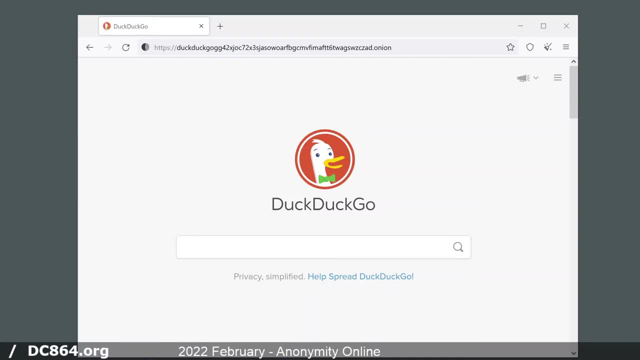 are options and services when it comes to your mobile devices, but because of the inherent insecure nature of mobile devices, they're designed to give away an identity, to have an explicit identity associated with them. Even if you're using burner phones, your ability 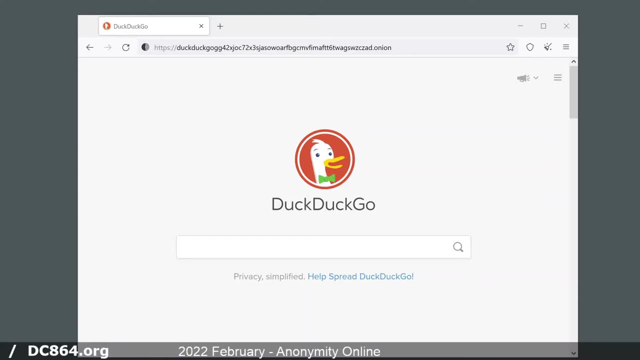 to abstract yourself from that is very limited. So recommendations if you're looking for them: yes, there's Warbot for Android, There's some services like that. Those are, you know, fine, but just realize, from an operational security standpoint it's nowhere close to. 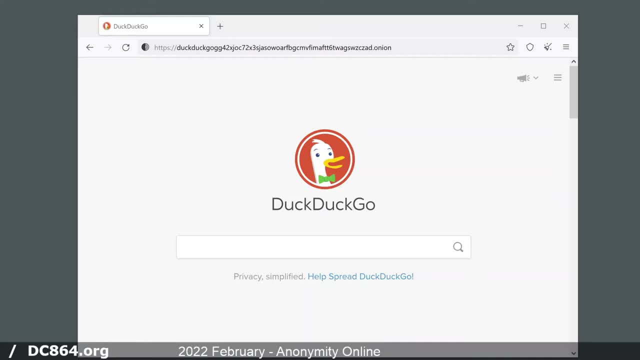 the same as running it on what you see here. now. They're very different And there's a ton of them in the Apple store. None of them are valid, None of them are legitimate. So like, basically, if you have iOS, just if you see Tor in the store, just know it's not. 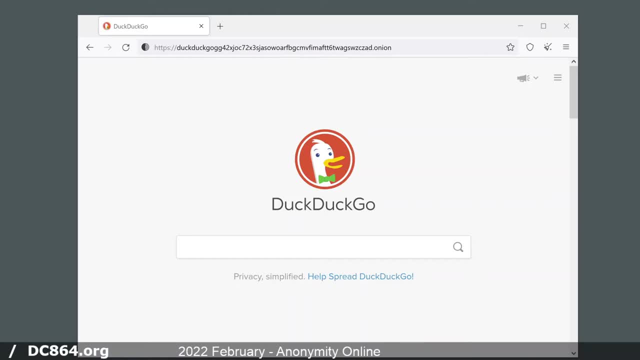 from the Tor project, you know. Skip that altogether. you know, Save your research or something else for later on. And the last thing I want to leave you with is this isn't just for security researchers, You know. I think about my family, who are maybe older. 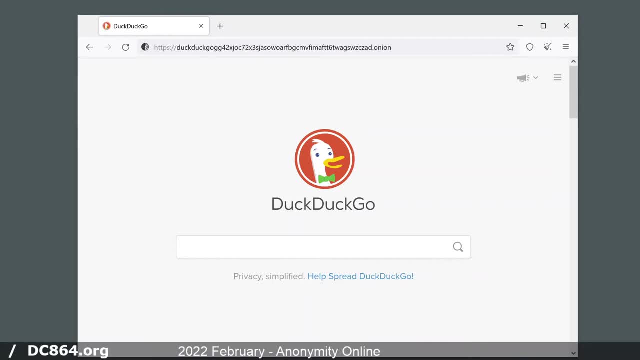 and some of them are doing research on health issues and stuff like that, and they are constantly getting phone calls about or advertisements that are, you know, basically like the old school pop-ups right Advertisements in their search history based on the problems that. 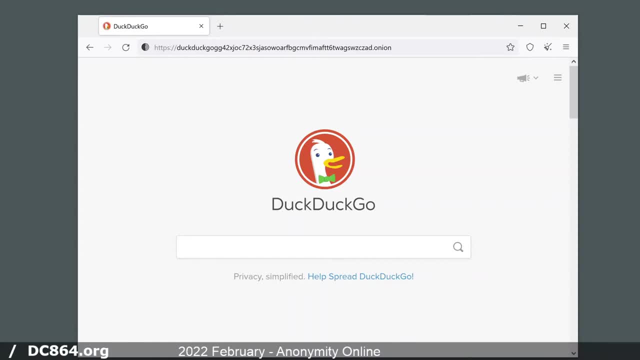 they're feeling that are very personal with their life. Share this with your family and friends, Not just because the more people using Tor creates a broader pool- for that you know all of us to hide in, but it helps prevent them from being exploited online as well. That's all I have for this week. 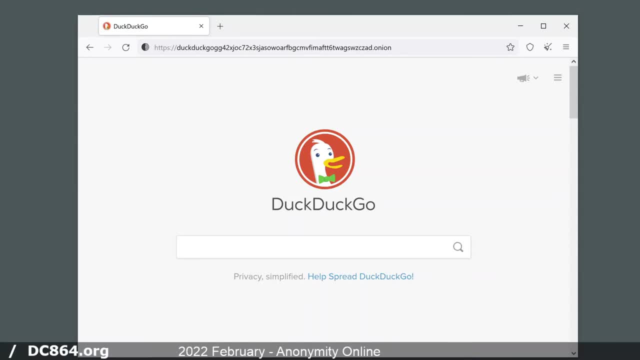 this month. You don't want to change the size of the browser, That's right, Yep. So it opens to a default size and you want to kind of leave it that way. They, you know that's a great point. They've calculated that to be the most standard and average across the. 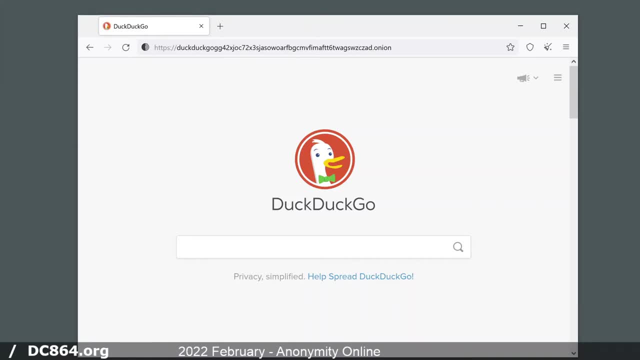 general populace. Yeah, we'll transition. If there's no other questions, we can do that, yeah. Yeah, I got a question- I had questions about color, but I'll save it for next week- Like: should we be using Tor for, like normal browsers? Should it replace Chrome? It depends. 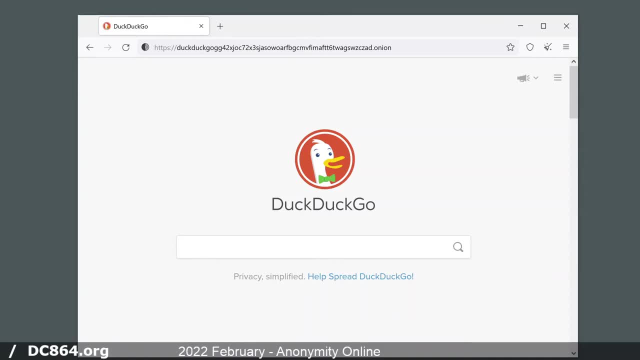 Like. that's an individual choice up to you. I advocate- yes, I think it should- as a default browser. I personally am moving further and further away from Chrome, partly due to the organization that owns and controls that code, even though Chromium underneath has now populated. 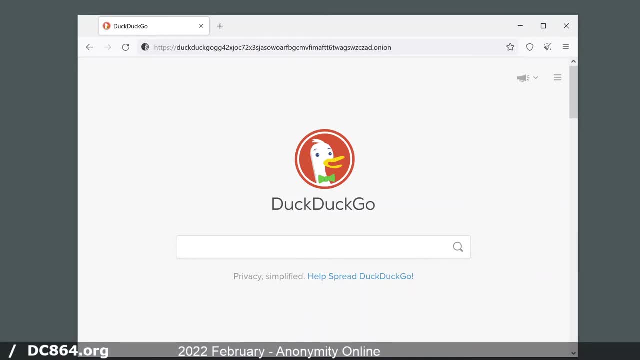 everything down to Edge and that's not. And the fact that it's also very heavily, it uses too much RAM. But you want to be careful with what you do inside the Tor browser because if you go to an account and log in, that service is still knowing who you are. You've just 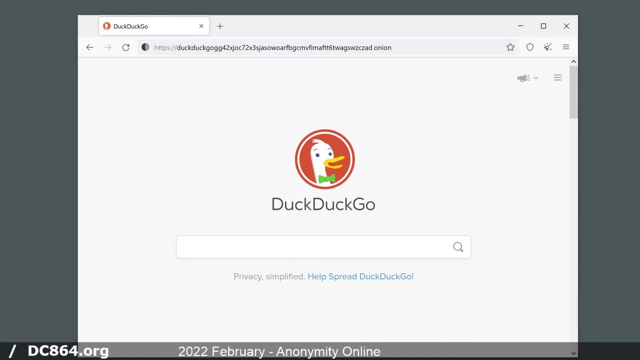 given up any kind of anonymity by logging into a service And what they know about you is they know that you're a Tor user, which is fine to a degree, because you're still not giving away your individual Like right now. if I were to disconnect from Tor and 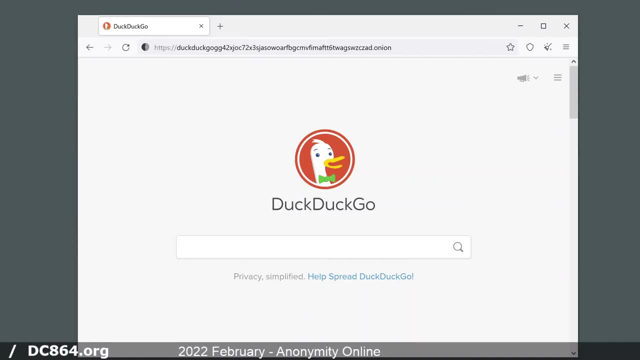 log into like a Gmail account, they would know end-to-end a lot of details about my asset and my account that I logged in with, whereas if you connect to Tor and you create a brand-new like ProtonMail account- Yeah, 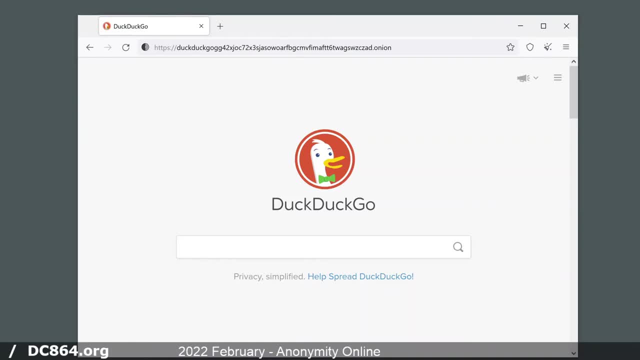 and you only ever access that ProtonMail account through Tor. like that's a pretty good OPSEC. The challenge becomes the minutia of the metadata. and did you one time maximize the screen, Yep? Were you logged into other tabs, into other services? Was any of the things being? 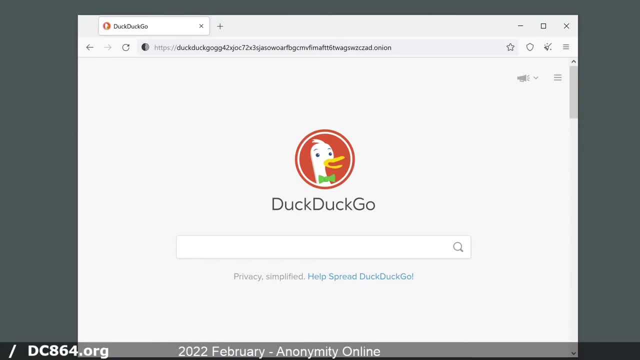 scraped. I mean, it was designed not to right, But the reality is is those types of things do happen and it's just a trail. So from like the OPSEC plan, like I got to intentionally use this browser just when I want to have that level of anonymity and 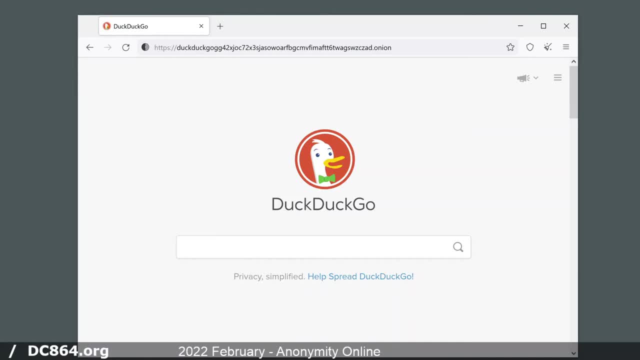 then I use other browser choices for day-to-day, with still a conscious effort to knowing that you know I'm being tracked, They know who I am, They know what I'm doing. I still use Firefox with no script and HTTPS everywhere, even though it's not Tor. but 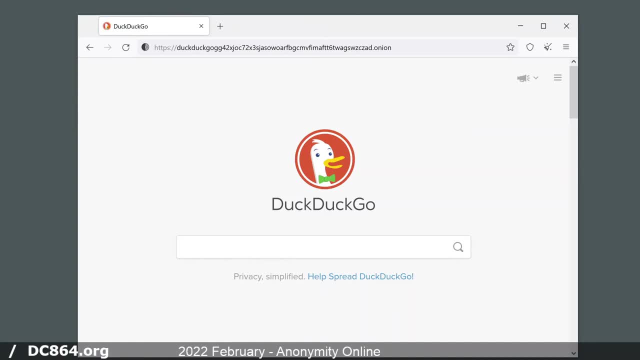 I kind of think of it as Tor Lite in a way. Do you mind going back to the slide that had the traffic routed? Yeah, I think that's an excellent way of explaining a threat model too, Like if I'm logging. 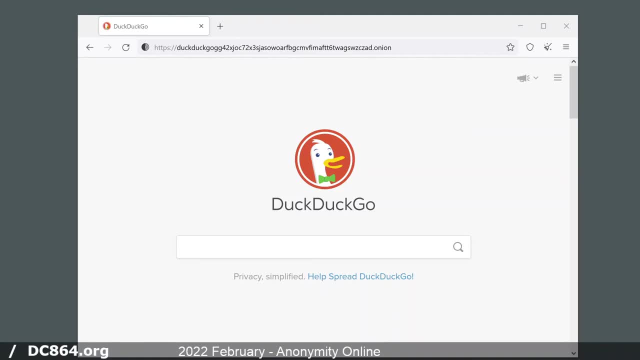 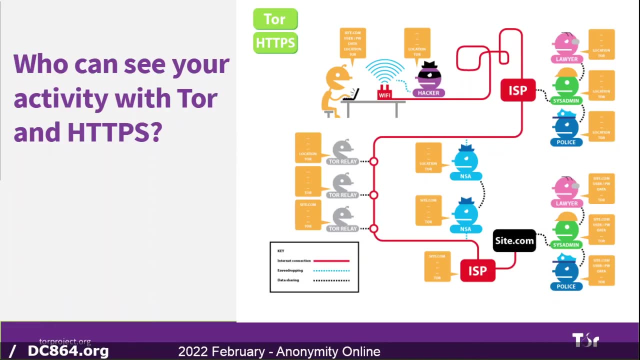 in with my bank account. all of those people already have that information to Tor. really, I'm going to use Firefox But yeah, Yeah, like all those people on the side already have bank account information as needed. But if I'm trying to do the security research, 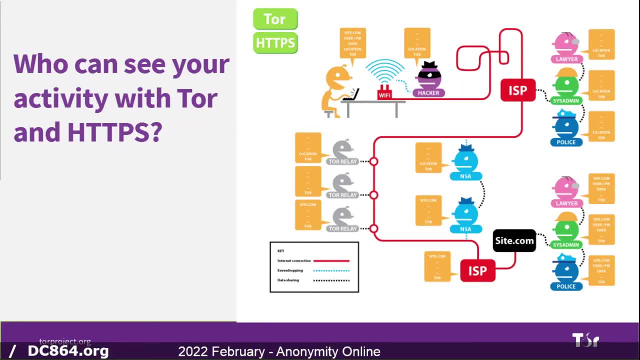 then they don't need to know that I'm going to go to Tor and boot that up. Yep. Next month I'd like to talk in-depth and show Tails versus Cubes versus Hoonix And personally, depending on the type of research. 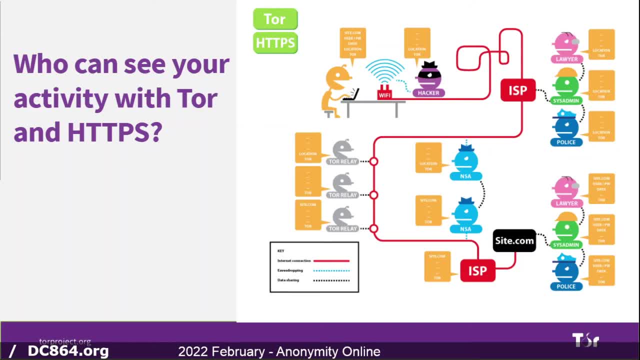 that I'm really diving into. I loved Cubes. I ran Cubes bare metal for a year And what I liked about it was it's really contained. Every single app and page that's opening up is isolated in its own sandbox and it detonates and can't go anywhere else or do anything. 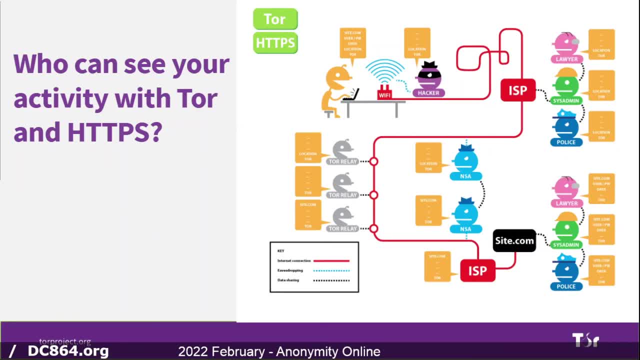 It's really slick And we've talked about it before in previous meetings, like back in 2019.. So doing this as a series and really just kind of stepping through logically how it all flows and connects together, I think would be helpful. So maybe next month we'll do. 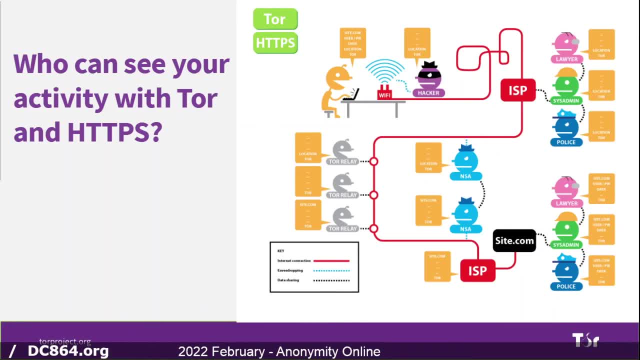 the abstraction. We looked at a browser, Then we'll look at isolating your OS And then we'll move into the network, the Tor network. Any thoughts about running Tor? your first hop through a VPN before you hit the Tor network directly from a browser, Because when you hit the Tor network your ISP still sees it. 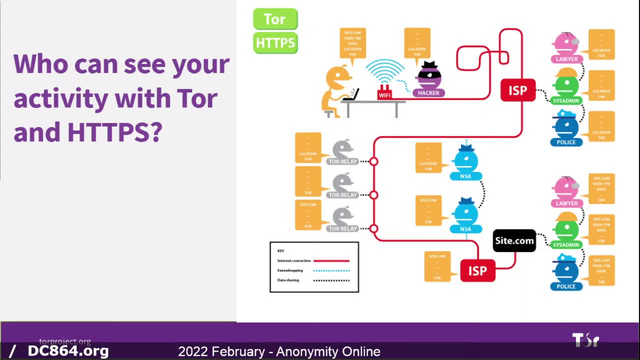 Yep Or sees that you are reaching out to that network And they, of course, can't see your tunnel. They actually have. I forget. I'm going to own that. I forget. That is on their FAQ. So they talk about VPN before Tor and VPN after Tor, or Tor plus VPN, Because that first and 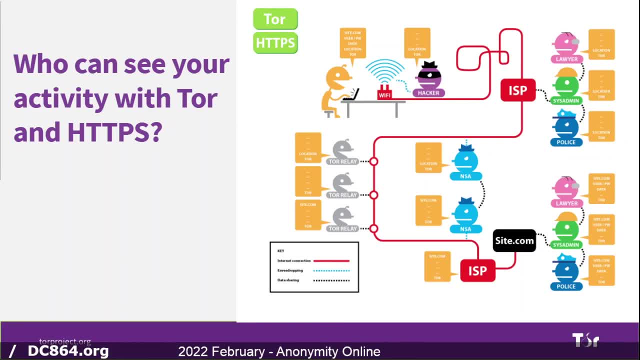 last leg are basically sitting in a little bit more of an exposed state, definitely an exposed state, And I can't remember. I think they advocated against it, but I can't remember which one it was. One was okay, one was not. So the rough plan, the idea- and I'm not trying, 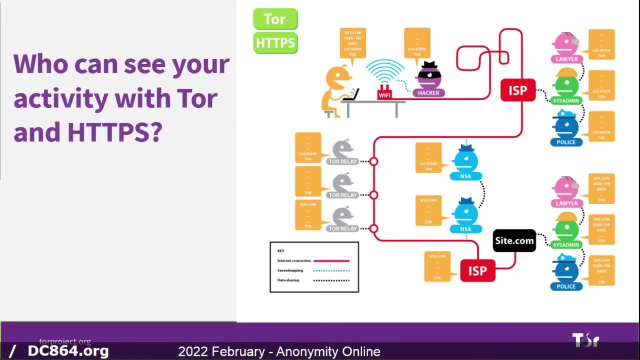 to commit you to anything. But the rough plan is we'll walk through this week looking at the browser, running the OS, running your own relays, your own entry node, your own mid guards, your own middle server. So guard is the first one middle server and exit node. You never run an exit node. 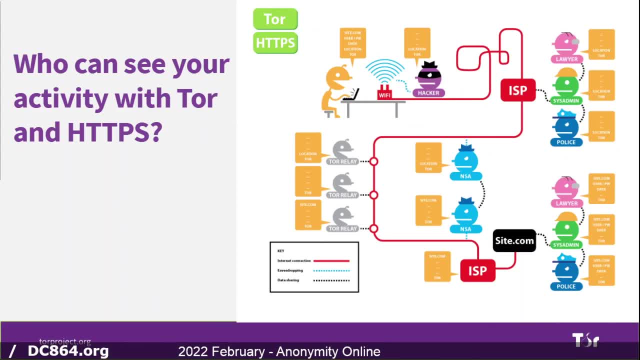 from your house, ever, ever, ever, ever, ever. And then we'll look at actually running a service on the other end of it And, if all goes well, knock on wood, fingers crossed, we're going to put together and publish how to build your own Tor network. 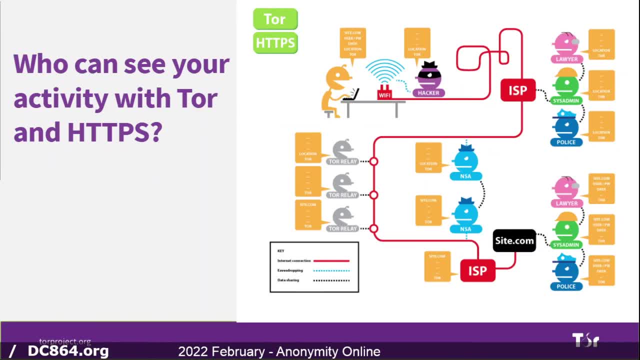 And like in our Workstation or VirtualBox, with your own service on the other end that you can control and play with. So that's you know, given time, if we could work it out. we're playing around with how that can look. 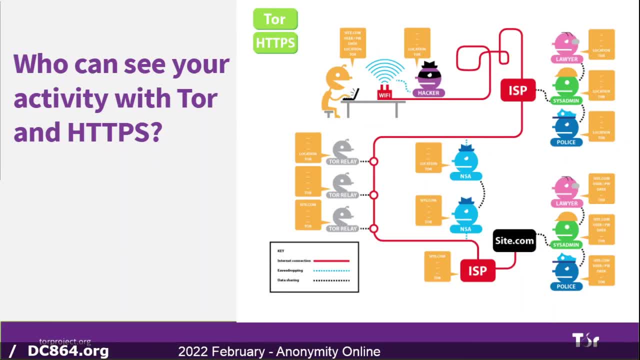 That's the plan, So you could host your own service on the Tor network and access it. Yeah, of course Not from your house, From your house, not my house. Yeah, the neighbor's WiFi for that, And there's two services we're looking into that. There's actually a link to the. 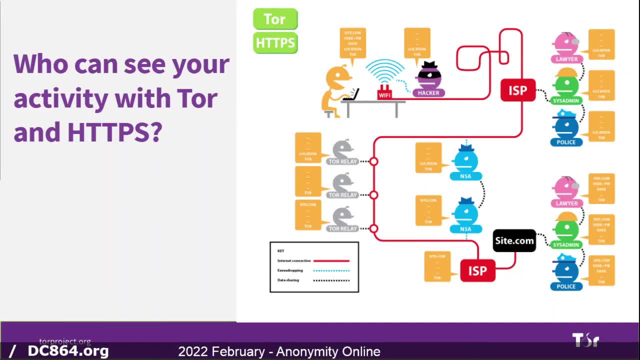 Tor network And that's for the Tor network. So if I go to Tor network, if I go to Tor network, an onion share service that we're going to stand up, that you can do. It has a really cool feature and I know I'm trying to get spoilers right now. 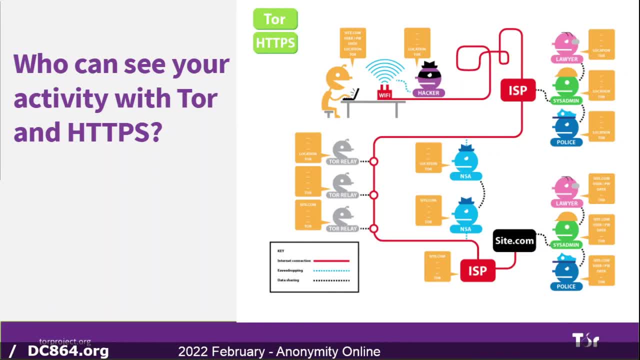 but it's kind of like Boxcom or Dropbox and one of the options you can set when you put a file in there is stop sharing as soon as it's downloaded the first time. So you get an immediate log entry that so-and-so downloaded this. 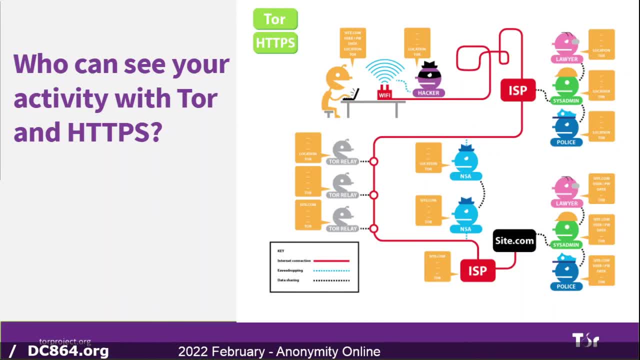 sharing is disabled at this point. Pretty slick, And then maybe run it as a run your MUD client through it. MUD game- I'll do my research. I don't know of any, So MUD is multi-dungeon. 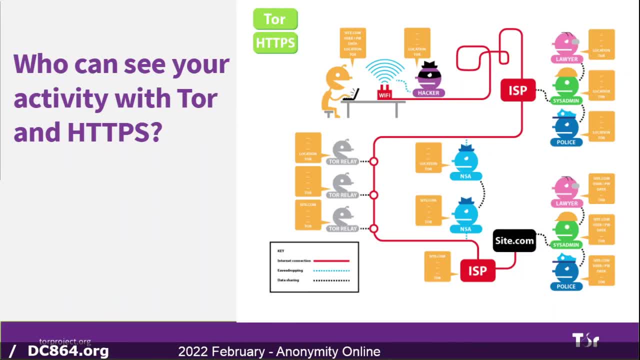 I don't know of any MUDs that are hosted and available on Onion. If you get it working, you're going to have to update your web page. I totally will. It's a claim to fame: We are one of the oldest running MUDs.